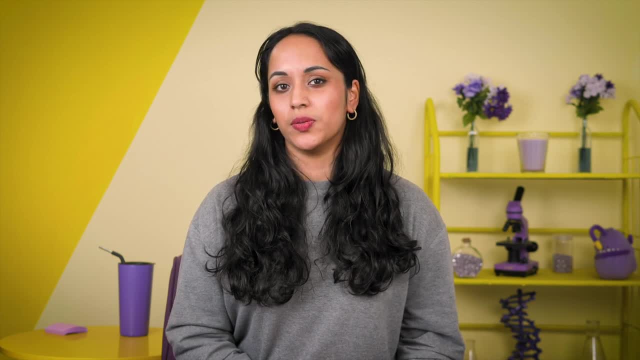 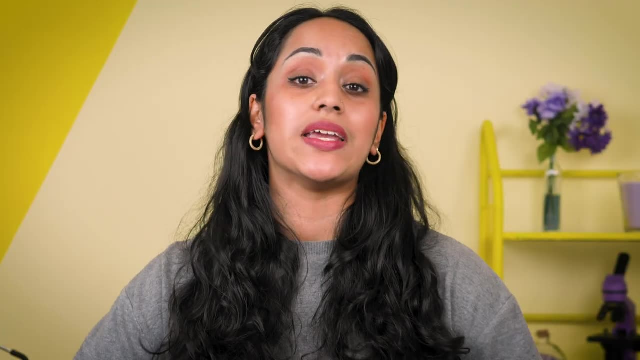 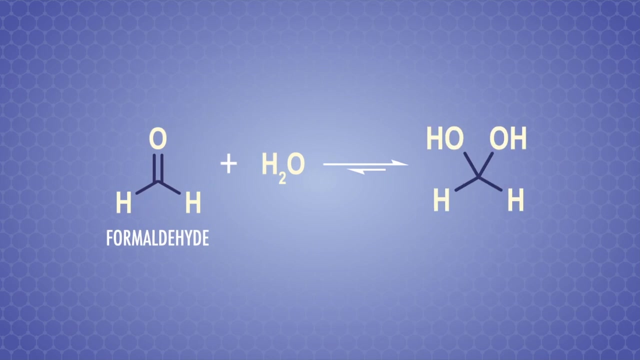 And other nucleophiles can also attack the carbonyl group. In this episode we'll focus on addition reactions of oxygen and nitrogen-based nucleophiles. A simple oxygen-based nucleophile that we're already quite familiar with is water. If you mix water with an aldehyde or ketone, an equilibrium forms with a hydrate form. 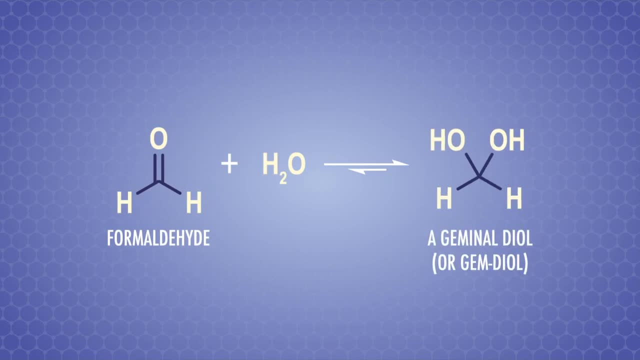 called geminal diodes. The word geminal is similar to geminis, one of several Latin words describing twins, And in chemistry geminal is used when we're talking about a molecule with two or more of the same functional group attached to a single atom. 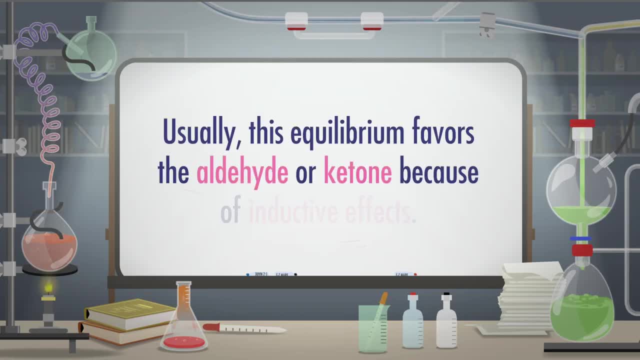 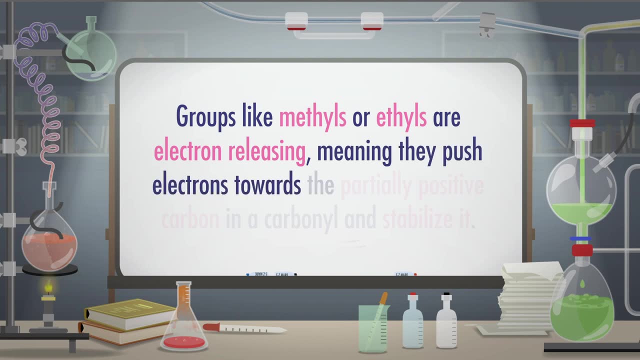 Usually, this equilibrium favors the aldehyde or ketone. because of inductive effects, Groups like methyls or ethyls are electron-releasing, meaning they push electrons towards the partially positive carbon in a carbonyl and stabilize it. There are examples that break this pattern. 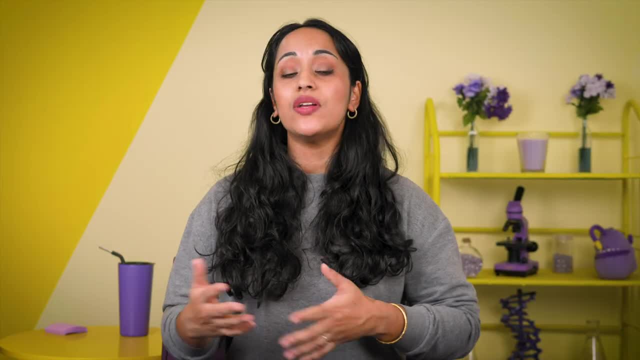 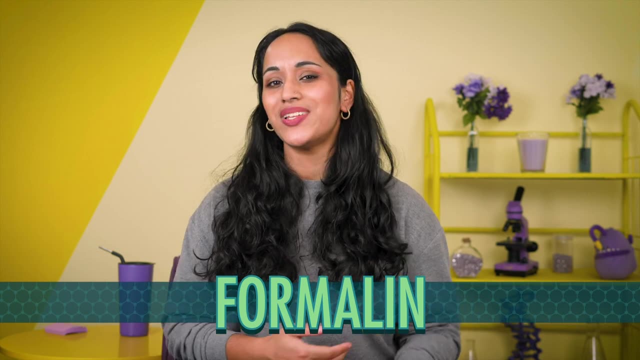 though, like the smallest aldehyde, formaldehyde. Mixing water with formaldehyde produces a solution called formalin. Formalin helps preserve tissues from decay, so it's what scientists use to preserve tissue specimens in jars. And not just scientists: artists too. 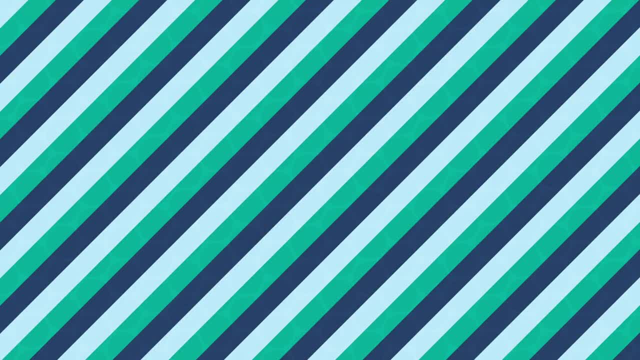 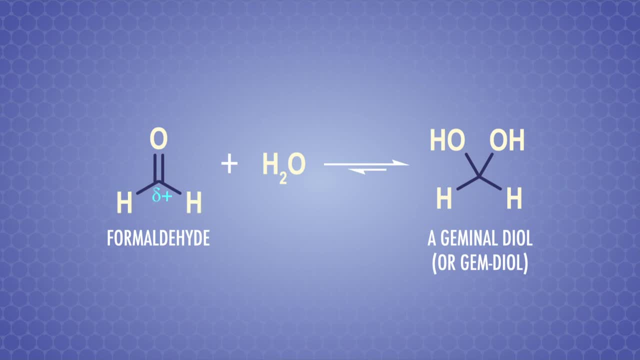 Damien Hirst exhibited a whole preserved tiger shark, Thinking about inductive effects. the hydrogen atoms on formaldehyde don't do much to stabilize the partial positive charge on the carbon, So the equilibrium in a formalin solution very much favors the gem dial, not the aldehyde. 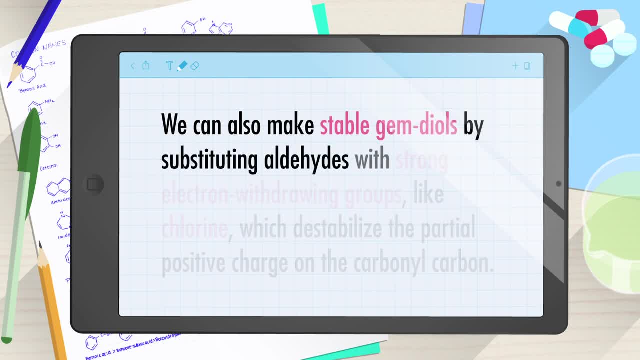 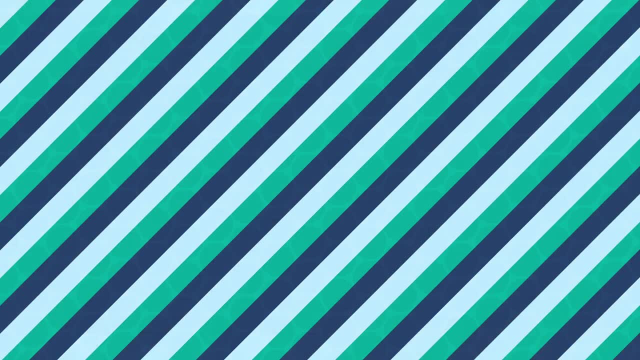 We can also make stable gem dials by substituting aldehydes with strong electron-withdrawing groups like chlorine, which destabilize the partial positive charge on the carbonyl carbon, For example, if we mix 2,2,2-trichloroacetaldehyde with water. 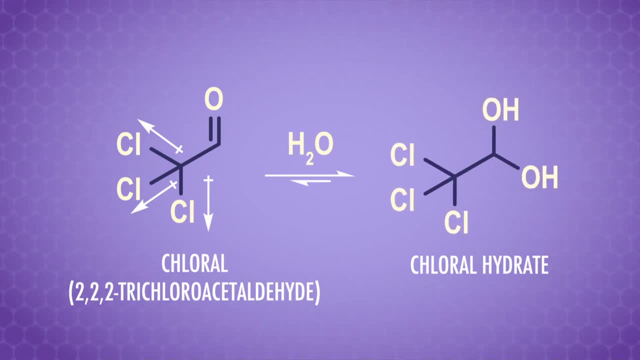 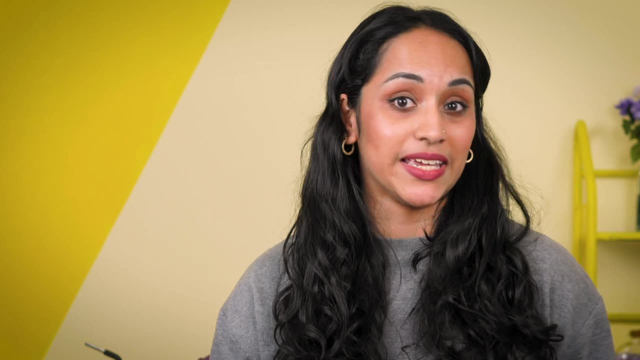 it forms chloral hydrate, which was given as a sedative in asylums and much abused in the late 19th century. Chloral hydrate in ethanol is colloquially known as knockout drops or a Mickey Finn, which is probably named after a Chicago bartender who gained 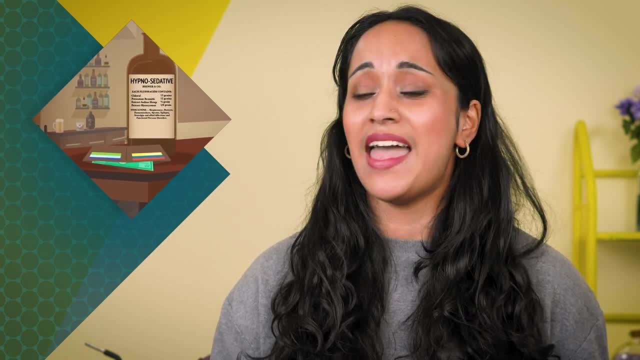 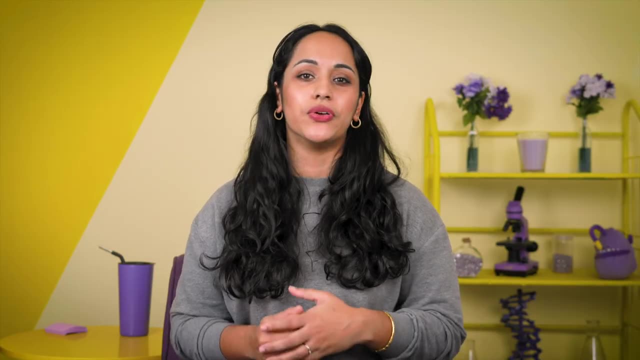 infamy after using this mixture to incapacitate and steal from some of his customers. Big yikes. Now we can also react carbonyl compounds with other oxygen-based nucleophiles like alcohol groups. When a single alcohol group adds to an aldehyde, we get a hemiacetal. 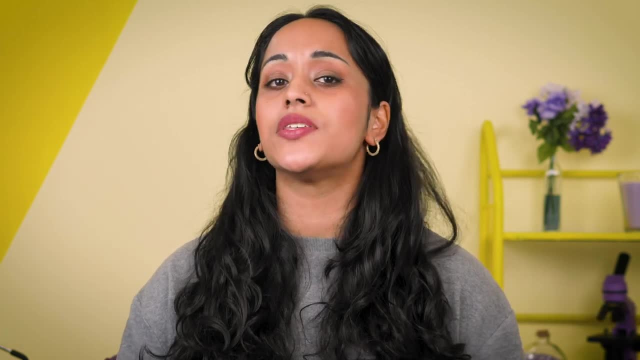 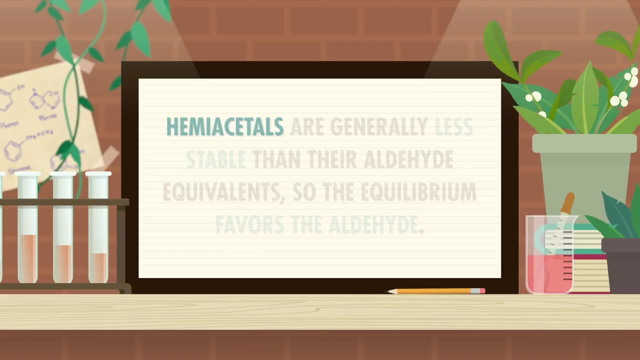 The name comes from the Greek word hemi, meaning half, because only one alcohol is added. There are also full-blown acetals that we'll talk about in a bit, which have two alcohol groups and they're called hemiacetals. 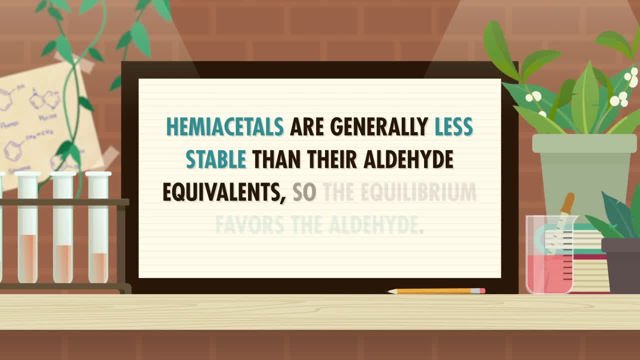 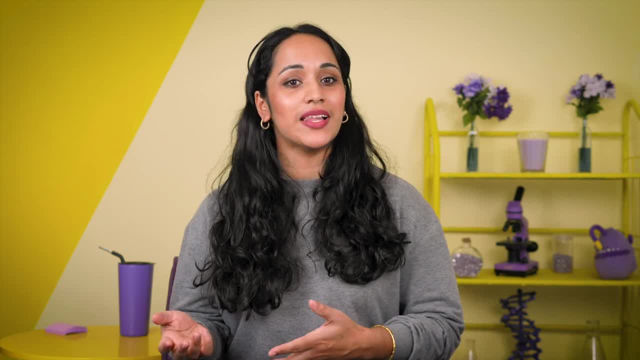 Hemiacetals are generally less stable than their aldehyde equivalents, so the equilibrium favors the aldehyde, as it does with many gemdials, Sugars and other molecules that can form intramolecular and cyclic hemiacetals can be exceptions. 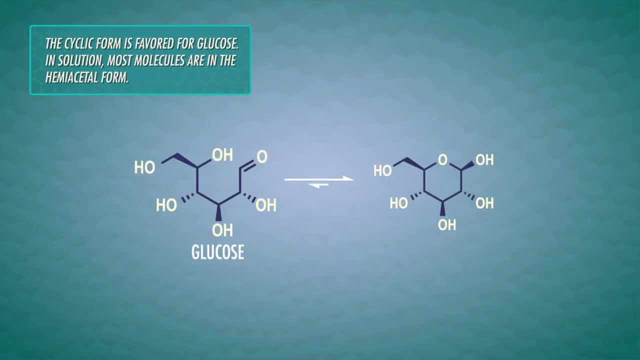 In aqueous solution, glucose rapidly interconverts between its straight chain and cyclic forms when one of its alcohol groups attacks its carbonyl carbon, Since the carbonyl group in glucose has a trigonal planar geometry. and our intramolecular hydroxynucleophiles? 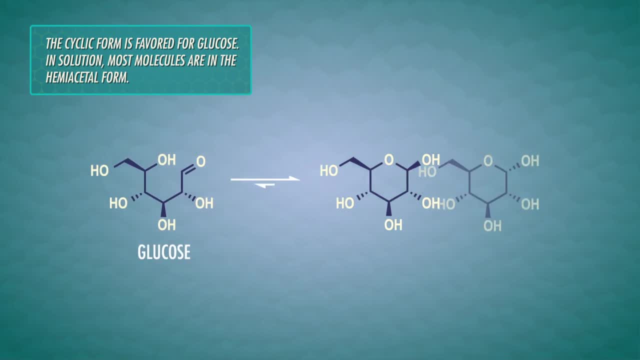 can attack from either side. our hemiacetal products are two diastereomers, But we can get even more specific in what we call them. The sugar world actually has lots of special vocabulary. The hemiacetal carbon of a sugar is called the anomeric carbon. 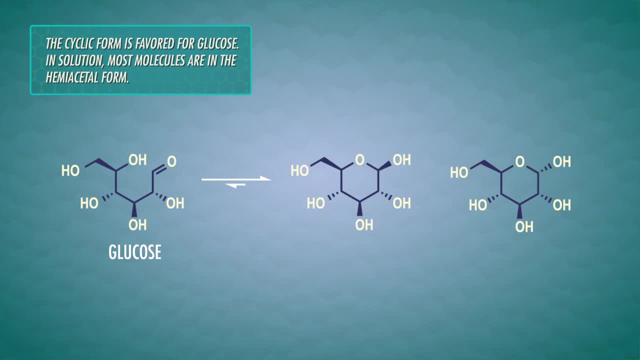 So these two products are more precisely called animers, one labeled alpha and one labeled beta. In the beta animer these groups end up on the same side, and in the alpha animer these groups are opposite. The beta animer of glucose is actually favored in water. 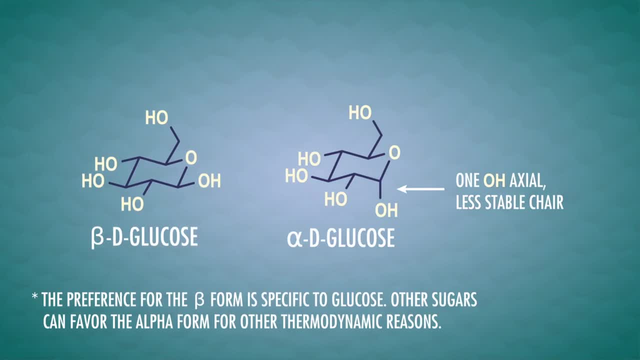 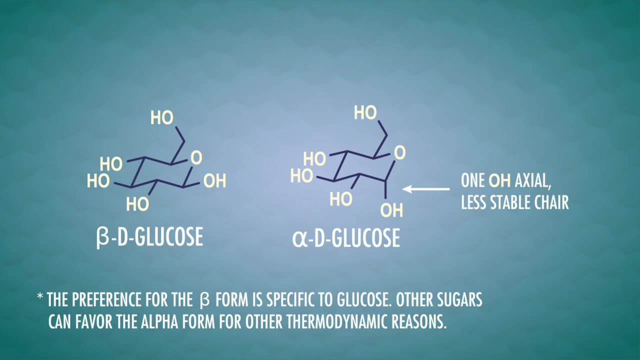 because, similar to cyclohexane, it can adopt a comfy, stable chair conformation And all the groups are equatorial, which also helps reduce steric hindrance and increase stability. That covers the basics of hemiacetals. 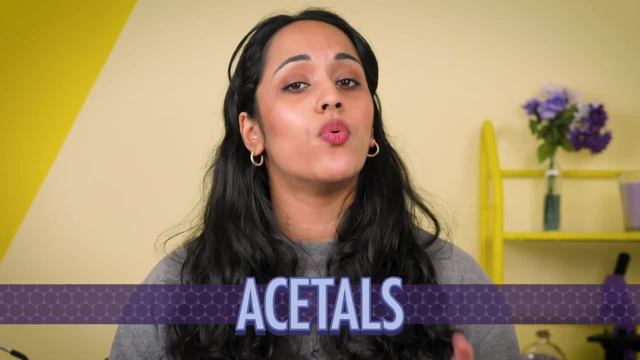 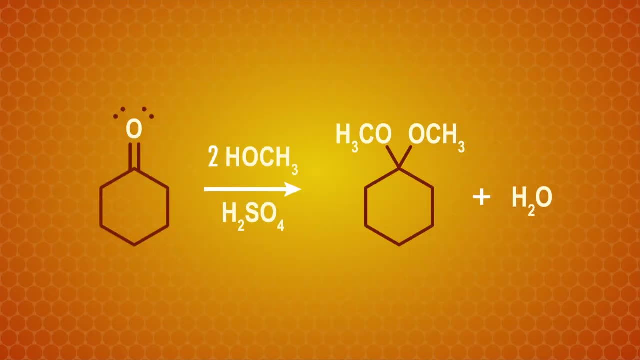 So now let's take off that hemi prefix and make acetals, which form when two alcohol groups add to an aldehyde or a ketone. These reactions are acid-catalyzed, so the three players are a carbonyl group, an alcohol and acid. 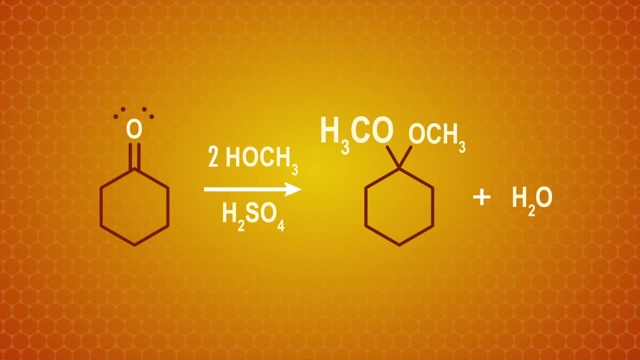 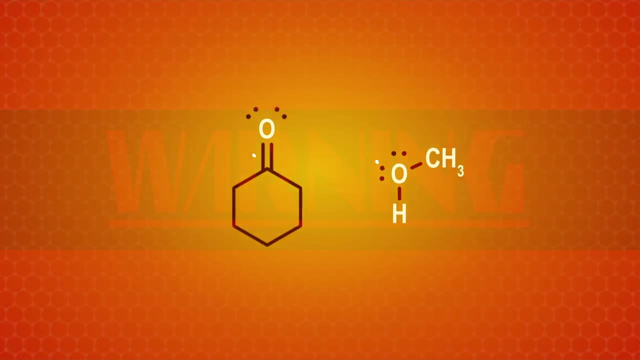 Looking at the summary reaction, we can see that we need to add two molecules of methanol to the carbonyl carbon to form the product. So let's puzzle through the mechanism. If we added methanol as a first step, that would give us a negative charge. 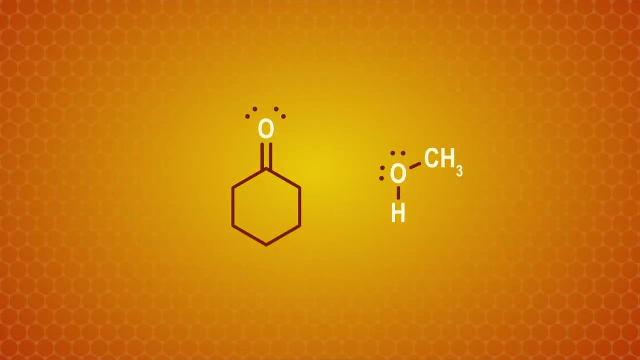 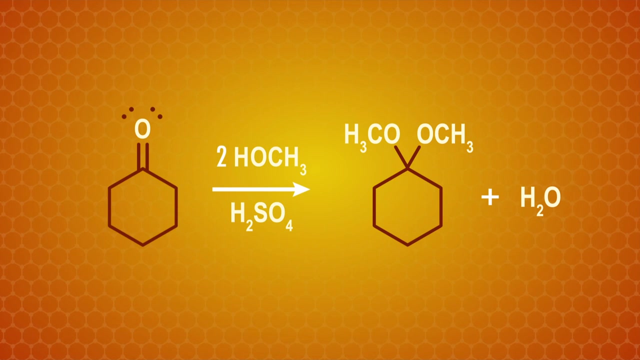 which we can't have in an acid. Okay, so we've gotta try something else. to start, In acidic conditions we have protons and there's a lone pair on the carbonyl oxygen. So what if that lone pair grabbed a proton from an oxonium ion? 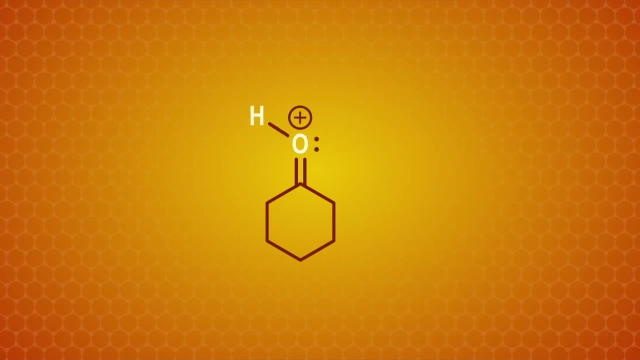 We'd have a positive charge, which is totally fine in our acid. Even though this works, we don't have a negative charge. So what if we added methanol as a first step? The oxygen isn't happy about this whole positive charge situation. 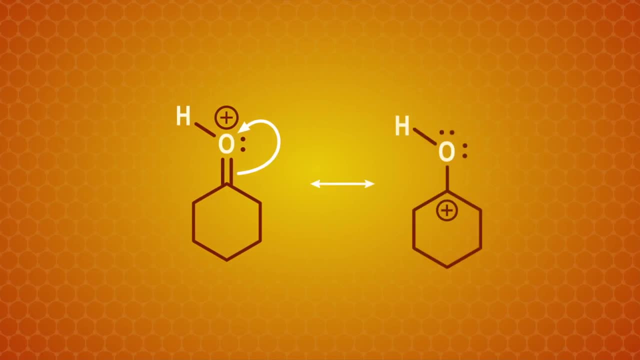 It draws a pair of electrons in the carbon-oxygen double bond towards itself, making the carbonyl carbon very electropositive and prone to nucleophilic attack. Looking at our product, we want to add methoxy groups to that carbon. 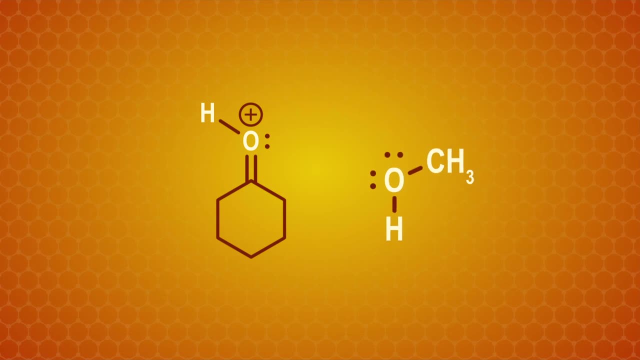 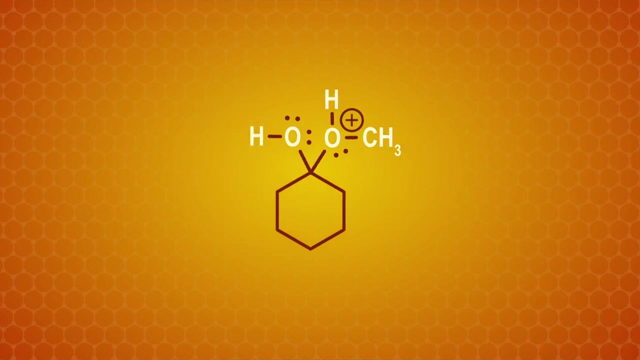 So that means the nucleophile we choose for this attack is our alcohol. Specifically, a lone pair on the oxygen of one of the alcohol molecules attacks the carbonyl carbon and adds a methanol. We've still got a positive charge. so this isn't stable enough to be an end product. 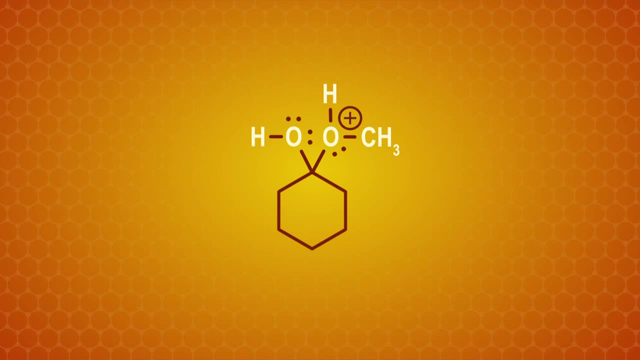 We've got to make our way to a neutral molecule somehow. Remember, we've got plenty of alcohol molecules floating around with two lone pairs on their oxygen atoms. So one of those alcohols can grab the spare proton on our molecule, leaving us with an OH and an OR group attached to the what-was-a-carbonyl carbon. 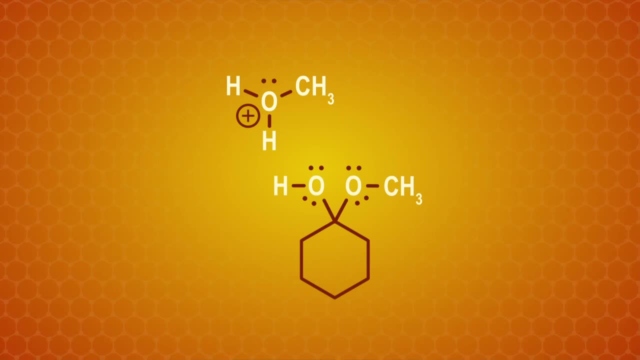 Now we have a hemiacetal, so we're getting closer. But to have a full-blown acetal we need another methoxy group. instead of that OH, In our acidic conditions we have a carbon-oxygen molecule, which is a carbonyl carbon. 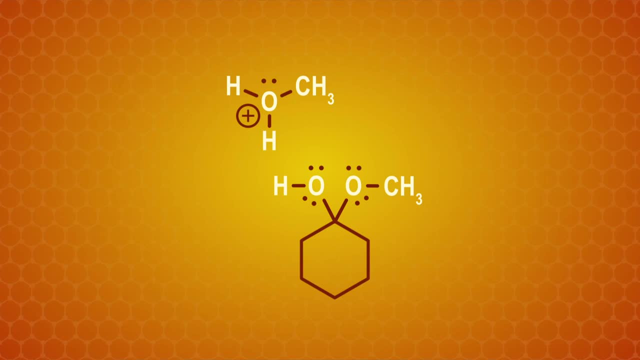 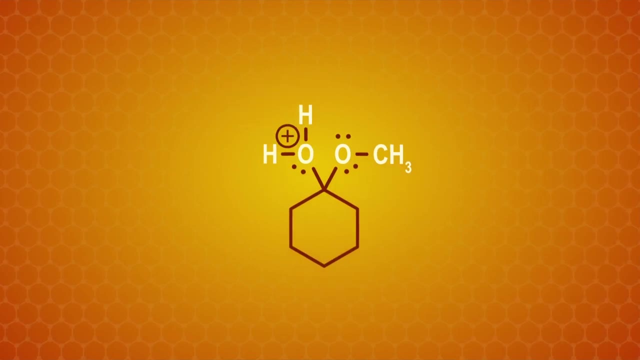 In our acidic conditions. we can get rid of the OH by making it a good leaving group. That OH grabs a proton from a protonated molecule of methanol. We might be tempted to have another molecule of methanol attack and kick off water at this point. 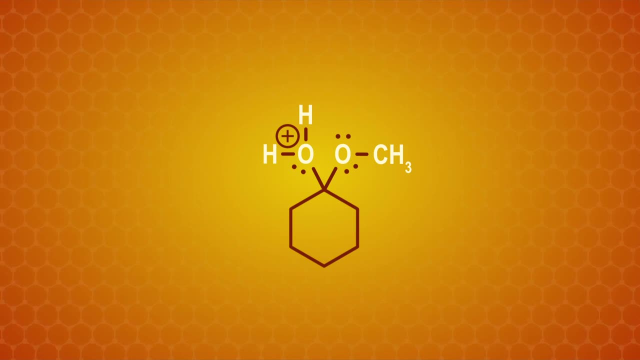 but that would be like SN2 at a tertiary carbon, Which doesn't work because, remember, there's not enough room for the backside attack. Instead we get a little help from the adjacent oxygen. A lone pair of electrons on the oxygen of the newly attached alcohol group help push out water. 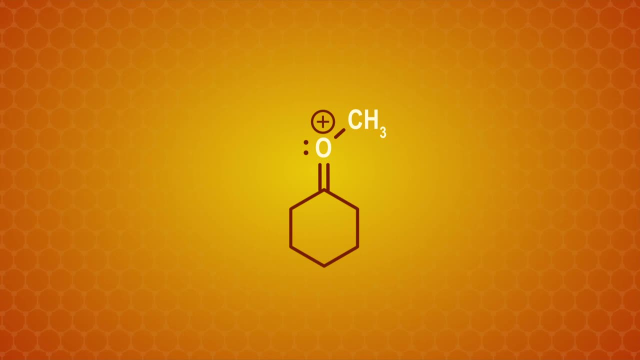 forming an oxonium ion and a molecule that's… not that different from where we started, Except now, instead of a protonated carbonyl, we have a carbonyl attached to a methyl group on oxygen. The similarity is important to notice, because we can basically do the same set of moves again. 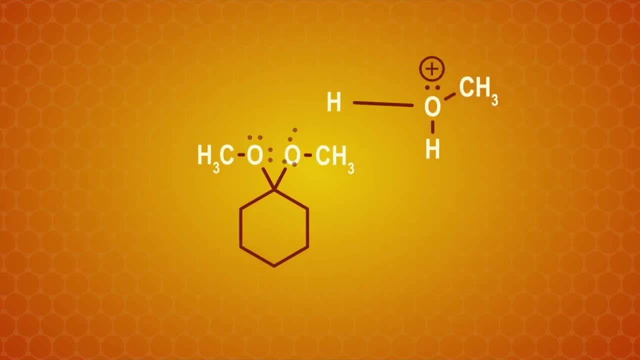 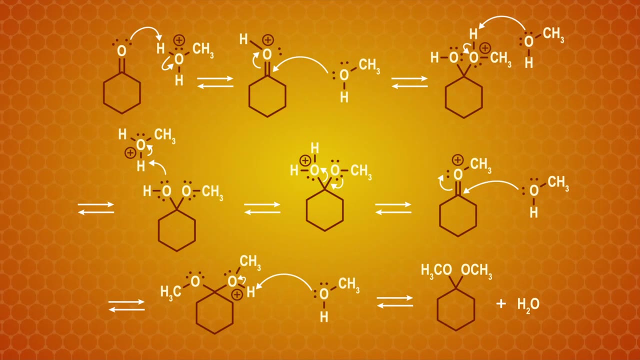 A nucleophilic attack from another alcohol molecule, followed by deprotonation and we get our acetal with two methoxy groups. We're done. That was a lot, So let's review all of the steps of our reaction mechanism with the arrow pushing. 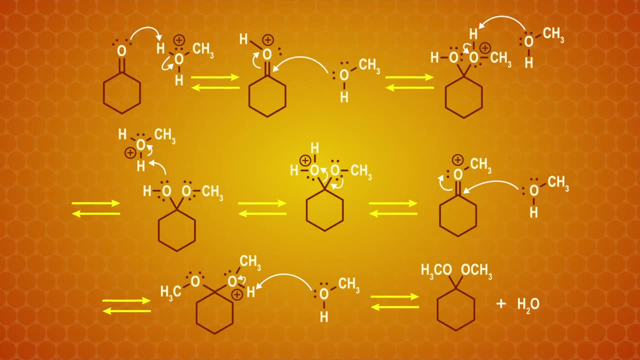 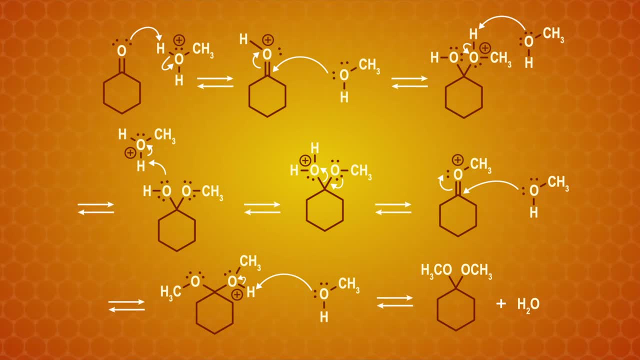 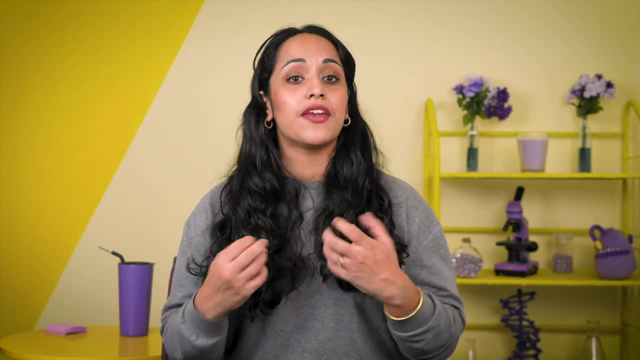 Heat an acetal with water, an acid, and boom Back to the ketone or aldehyde. But if acid isn't present, acetals are really stable once they're formed. In fact, they won't even react with really strong nucleophiles like carban ions. Acetal formation is an important strategy for controlling the reactivity of aldehydes and ketones in multi-step reactions, So we'll come back to this when we talk about protecting groups in a later episode. For now, we'll move on to another topic. 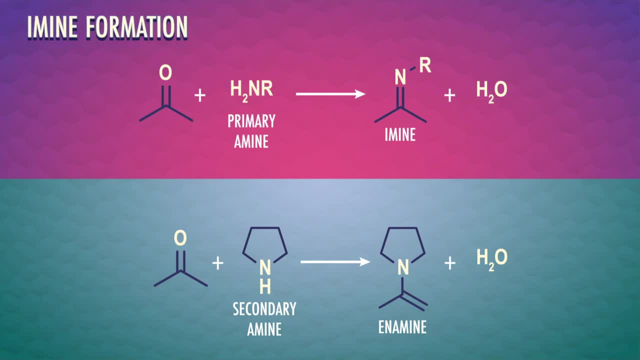 For now, we'll move on to another similar reaction involving the formations of imines and enamines. Immines are molecules with carbon-nitrogen double bonds, and enamines contain a carbon-carbon double bond next to an amine – an alkene plus an amine. 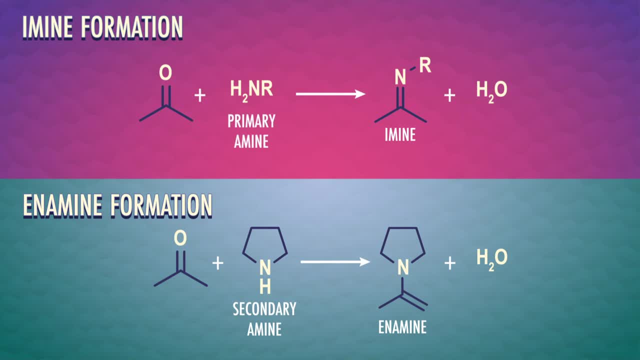 Immines come from a carbonyl and a primary amine, while enamines come from secondary amines. One way to remember the difference is to notice that the words imine and amine are the same except for one letter. 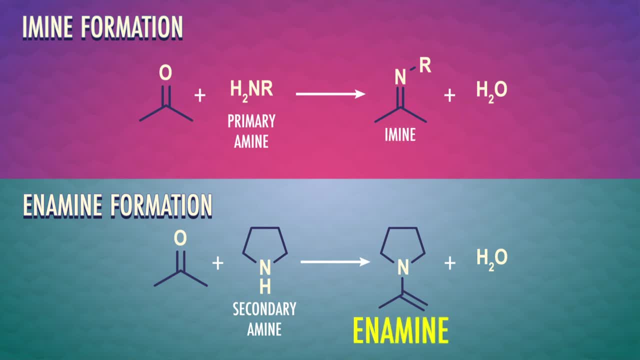 So imines come from primary amines. Inamine on the left is an amine and amine on the right is an amine. Amine, on the other hand, has two extra letters, so enamines come from secondary amines. 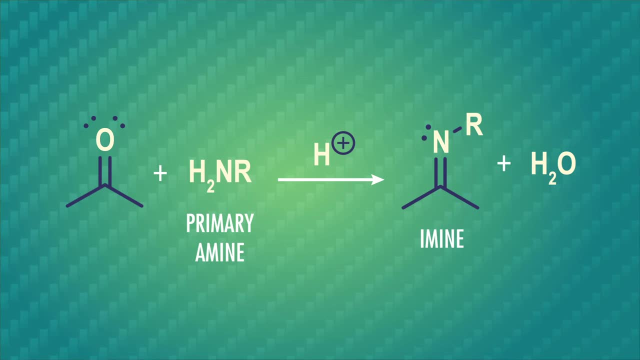 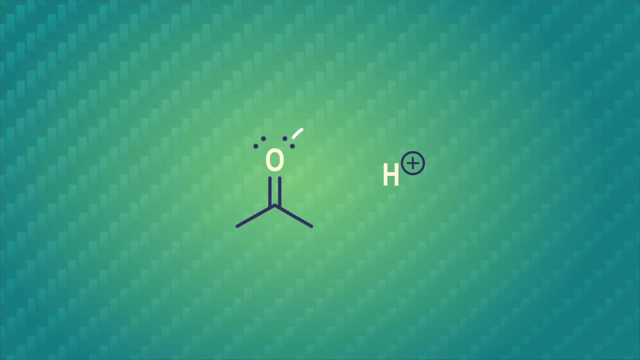 The mechanism for imine formation is similar to acetal formation, with three main players – a carbonyl group, a primary amine and acidic conditions. Once again, there's a lone pair on the carbonyl oxygen that can grab a proton. 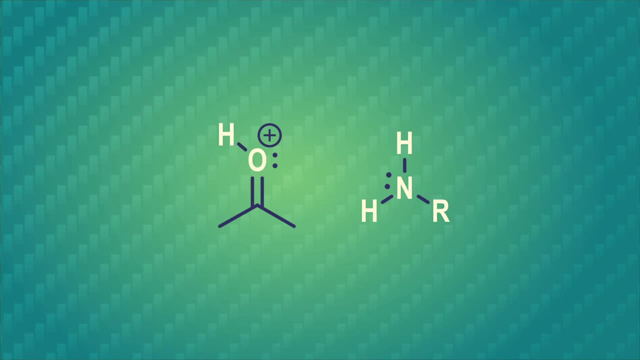 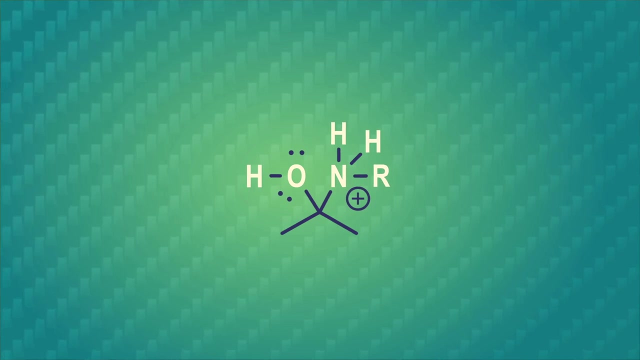 Then the nucleophile, which is the nitrogen in the amine this time, can attack the carbon atom of the protonated carbonyl group. The pi electrons in the carbon-oxygen double bond neutralize the axonium and our intermediate molecule has an amine and an OH on the what-was-a-carbonyl carbon. 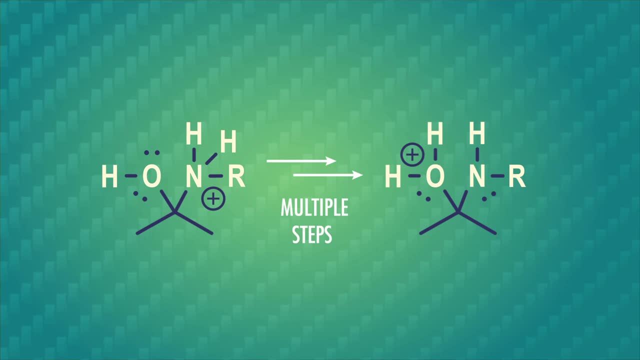 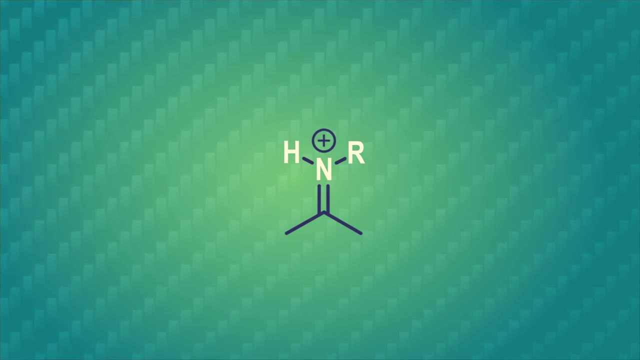 As in acetal formation, oxygen gets protonated, the nitrogen-lone pair forms a carbon-nitrogen double bond and water is eliminated. That leaves us with an aminium ion, which is any molecule with a positive charge on the double-bonded nitrogen. 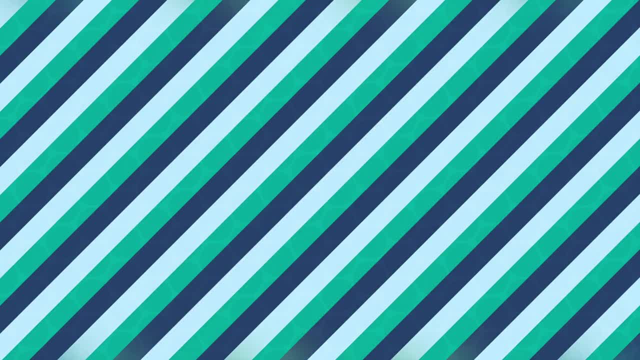 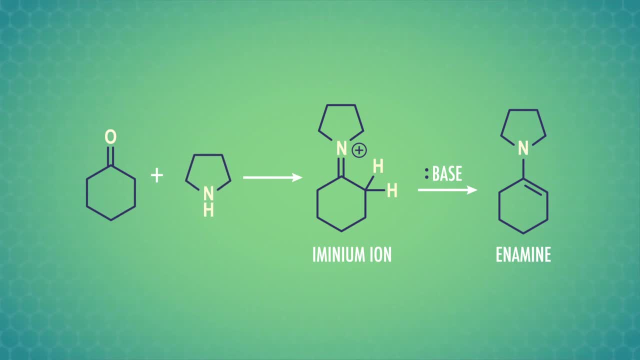 After a deprotonation we get an amine. However, if we're making an enamine and start with a carbonyl group, a secondary amine and acidic conditions, we can't do this final deprotonation step. 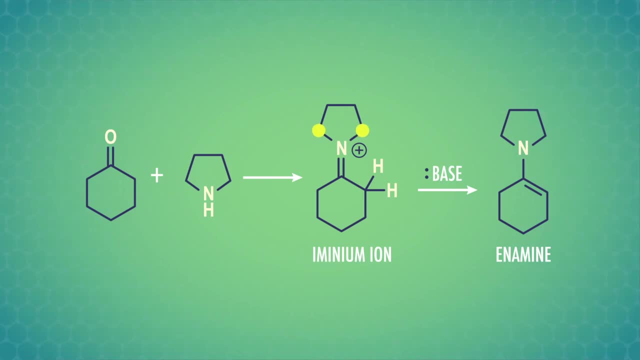 The nitrogen has two R groups instead of a hydrogen we can just kick out. So instead, the final step of the mechanism is deprotonating the carbon adjacent to our aminium ion, giving us an enamine. This is a great moment to mention a compound called ninhydrin. 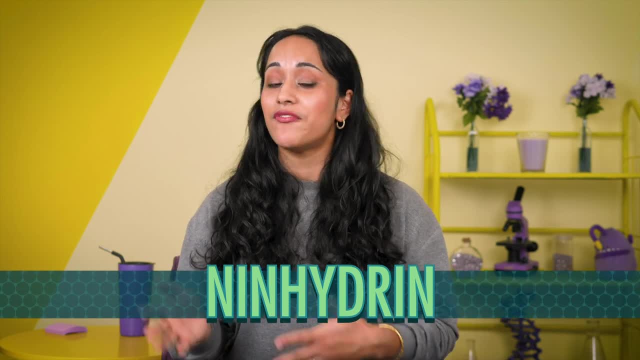 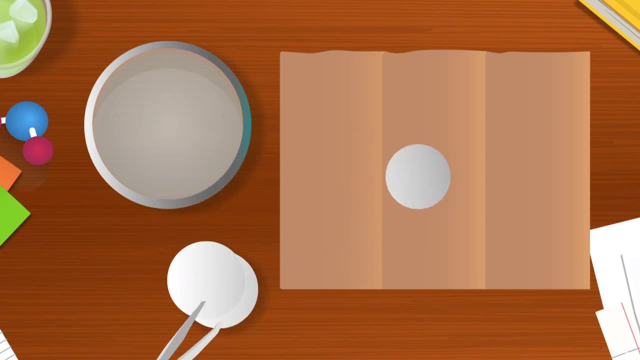 which is used in chromatography to identify amino acids and forensics to view fingerprints. Specifically, ninhydrin detects the amines present in the amino acids and proteins left behind by our fingerprints. When it reacts, it will detect the amino acids present in the amino acids and proteins left behind by our fingerprints. 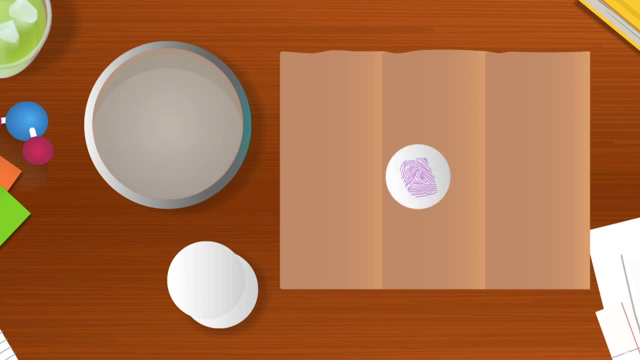 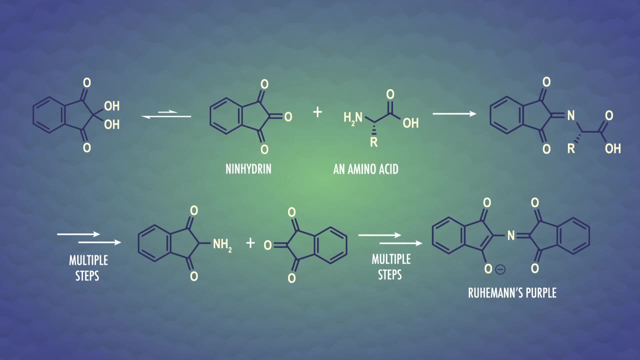 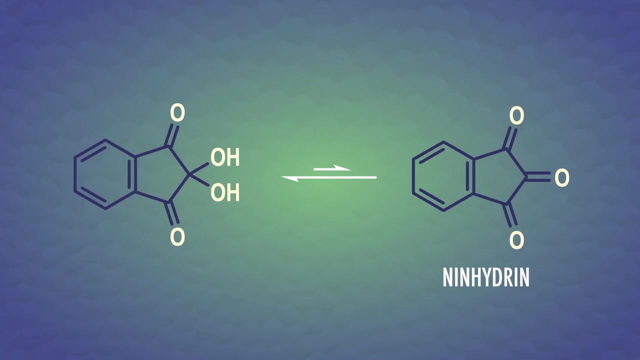 When it interacts with amino acids, a deep blue-purple color appears, called Ruhmann's purple. This is actually an amine-forming reaction that occurs on the keto form of ninhydrin, And the mechanism is fairly straightforward: That central carbonyl carbon in the five-membered ring smushed between all those carbonyl groups. 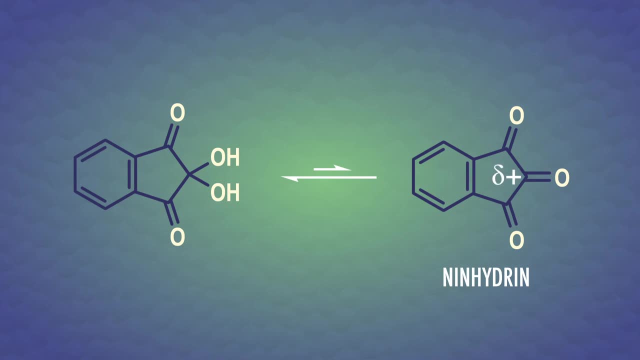 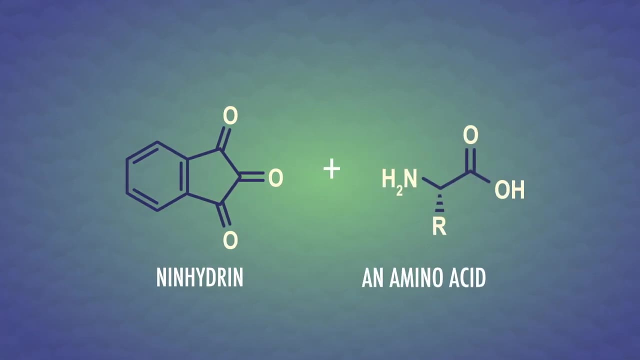 has a big partially positive charge, So it's really attractive to nucleophiles. As a result, when an amine turns up, say from the oily residue left by a finger, the lone pair on the right side of the ring is called a carbonyl. 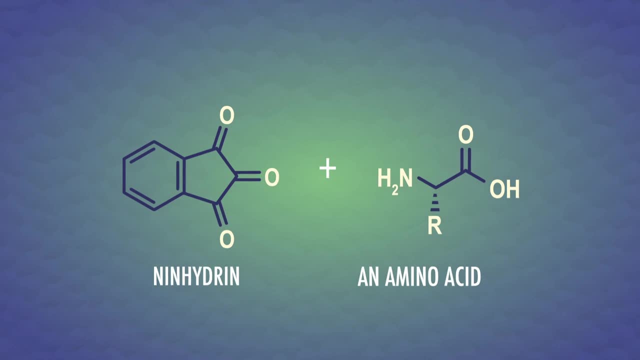 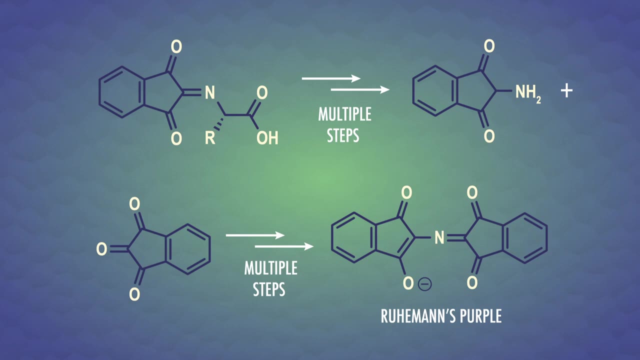 The lone pair on the nitrogen attacks the central carbon. Then the ninhydrin is dehydrated and we form an amine. The next few steps of this mechanism are beyond the scope of this episode, But basically another molecule of ninhydrin reacts. 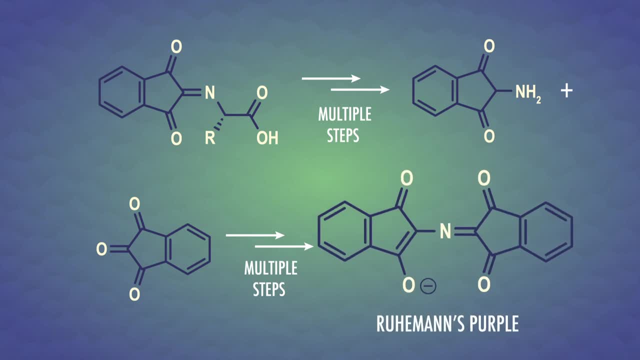 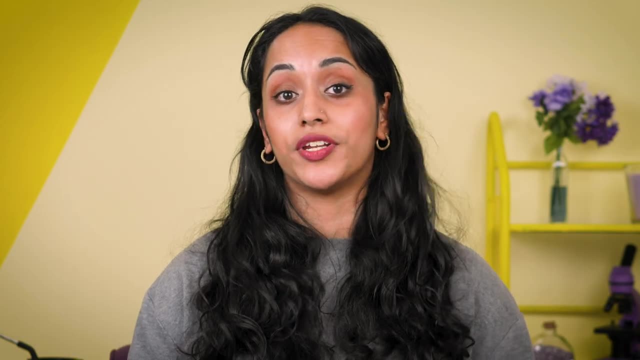 and the two molecules link up through the nitrogen atom. This compound is responsible for that pretty purple color and successful fingerprint sleuthing. To continue linking our carbonyl chemistry to real-world applications, we can also look at the anti-anxiety medicine – that stereotype of dramatic TV. 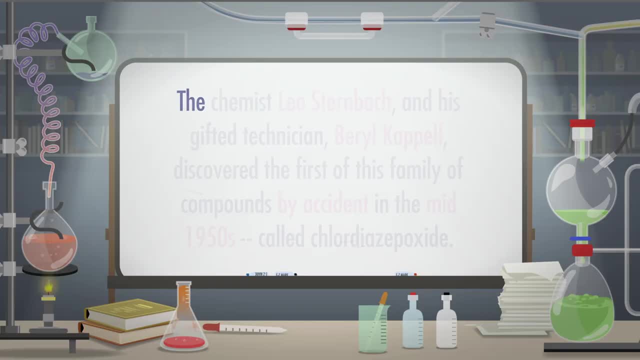 We talked about Valium to start, which is a brand name for diazepam. The chemist Leo Sternbach and his gifted technician Beryl Kappel discovered the first of this family of compounds by accident in the mid-1950s, called chlordiazepoxide. Kappel had been screening potential muscle relaxants for seven years when she found that this compound had anxiety-reducing effects. A few years later, the discovery of diazepam followed. These drugs quickly became popular because they reduce anxiety and tension without the knockout effect of something like chloral hyaluronate. 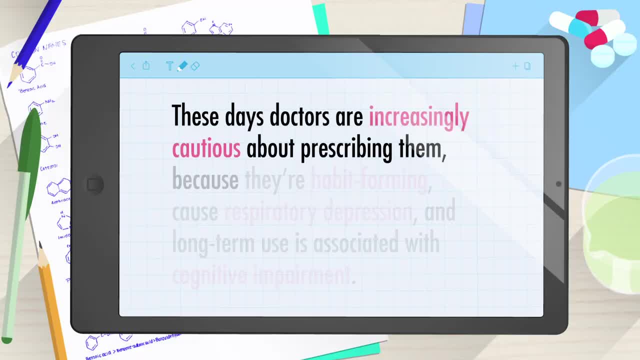 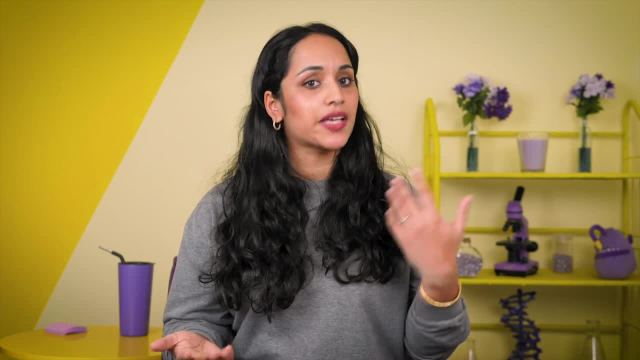 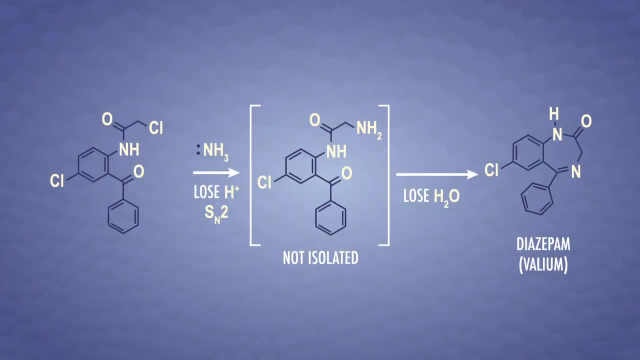 These days, doctors are increasingly cautious about prescribing them because their habit-forming cause respiratory depression and long-term uses associated with cognitive impairment. However, despite its complicated medical history, diazepam is a useful example for carbonyl chemistry. Let's focus on one part of its synthesis.